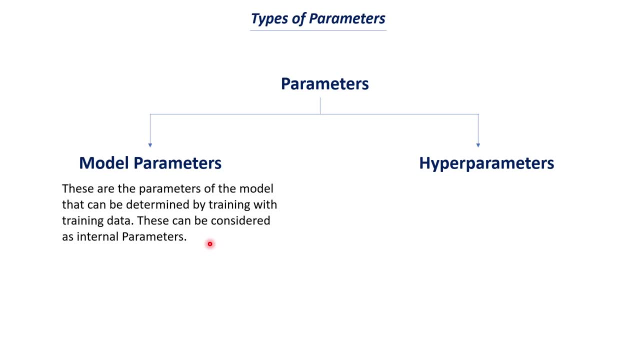 it will try to find the most optimum parameters. So these parameters that are determined by the model using the data are called as the model parameters. So once we, you know, carry out this training process, the model will try to find the best parameters. So examples of these model parameters are weights and bias. So if you consider a linear 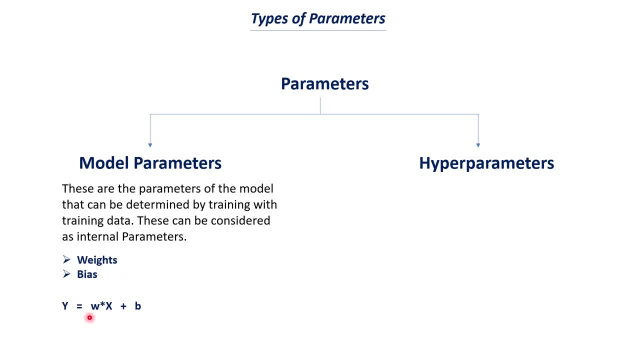 regression model. so we have the equations as: y it equal to w, x plus b, where y it a dependent variable. Okay, or you can call this as the target, and x it a independent variable. So if we consider an example, let's say that we want to determine what is the salary a person. 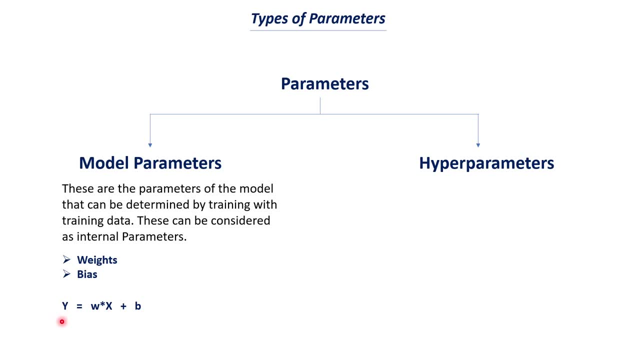 can make, depending on his years of work experience. In that case, y will be the salary that we are going to predict and x will be the number of y itself. So the erkennen we do a lot of of actual India in this case we are going to estimate, So the number at which, slightly 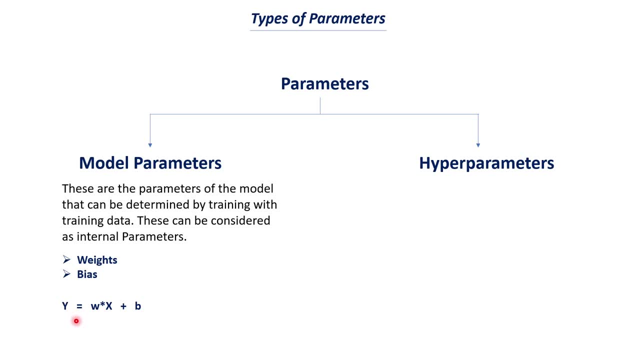 we calculate is that it will be he X plus and극 and in the, given that if, instead of the contribution, days of experience, okay. and we know that the equation of the line is given by y is equal to mx plus b, and here w is similar to the slope. so we know that we represent slope, as m right, and 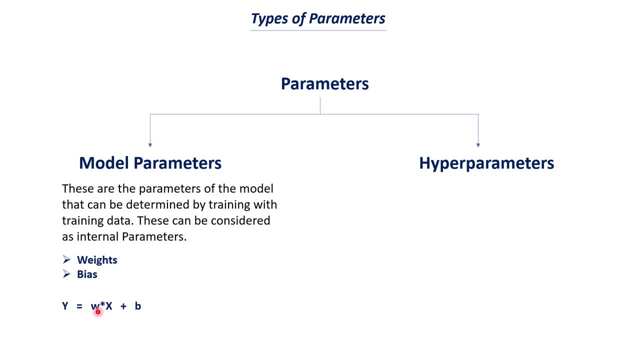 intercept as c, so instead of that we can write as w and b. so w represents your weight, which is similar to your slope of a line, and b represents your bias, which is again similar to the intercept of line. so this w and b will be your model parameters. okay, so we initiate with random. 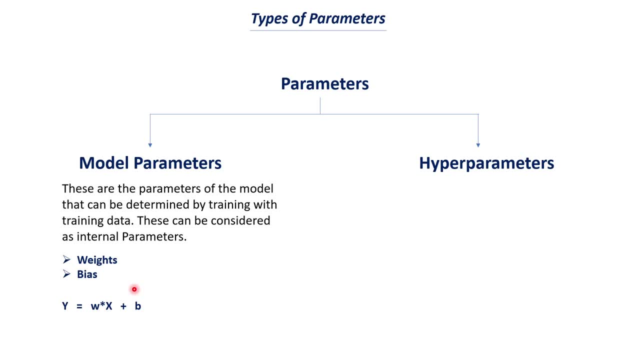 weight value and bias value and once the model is fit with the data, it will try to find which is the best parameter value for this w and b. so this set of parameters are called as the model parameters and there are other set of parameters called as hyper parameters. so hyper parameters are: 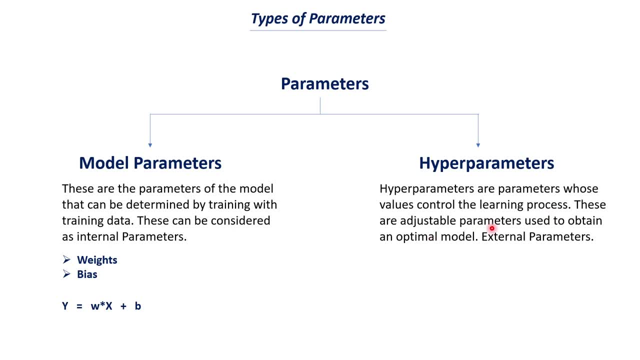 the parameters whose values control the learning process. these are adjustable parameters used to obtain an optimal model. so, and these parameters are also called as external parameters, so let's try to understand this. hyper parameters, as i have told you, these set of parameters, weights and bias, which we call as model parameters, are determined or these values are derived based 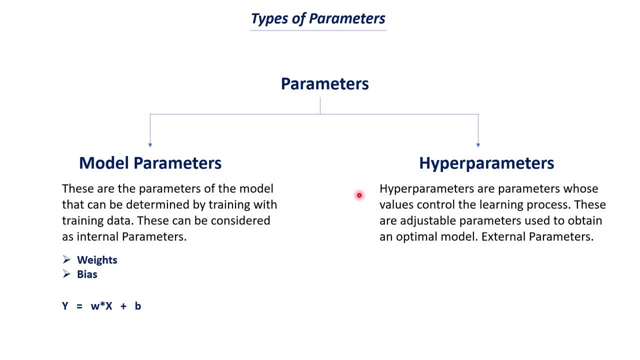 on the data set that we have. but the hyper parameters is something that you know we give to the model, so this hyper parameter determines how your model is going to perform. okay, so this set of values are determined by working on the data set, whereas this is given to the model, and 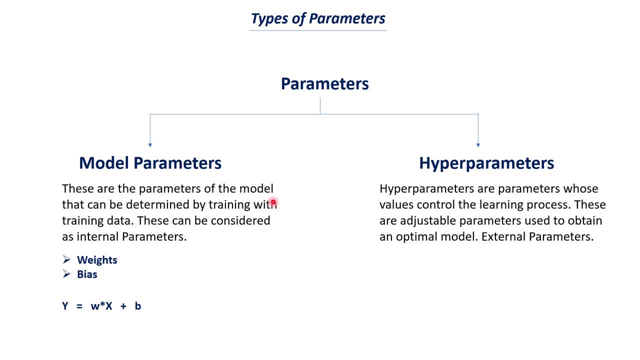 these parameters, you know, dictates our model is going to train from that particular data set. so hence we call this, call this as external parameters, because we can control the parameters. okay, so you can change the values of hyper parameters, but you cannot do it directly when it comes to the weights and bias, which we call as model parameters, because the model tries. 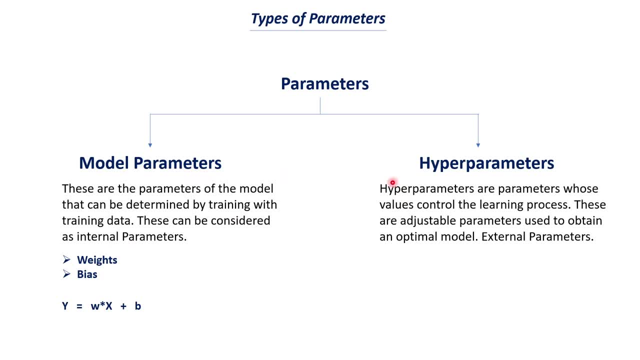 to find the best parameters on its own, whereas we control the hyper parameters. okay, and the examples of hyper parameters are learning rate, number of epochs and n estimator. so these are few examples. again, there are a lot more examples of hyper parameters. so learning, that is nothing but how. 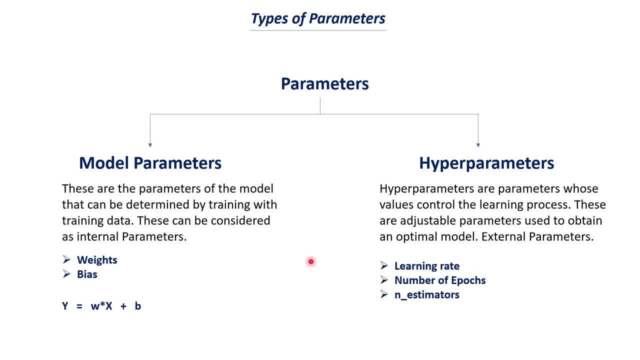 much do you want to change your weight and bias? so if you, uh, if you have seen my gradient descent videos before, so in that we have seen that, uh, when a model is training on a data set, what it will try to do is, initially, it will you. 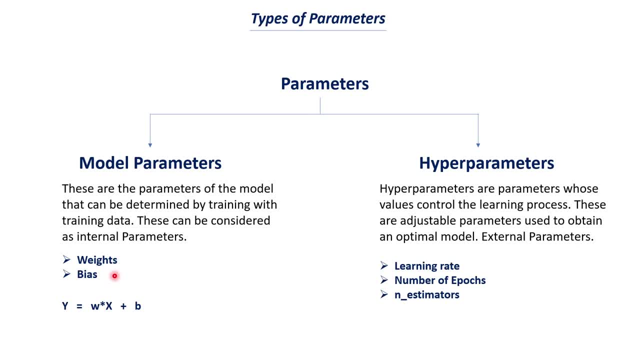 know, randomly assign some values to this weight and bias. so we usually initiate with you know value as zero. so after that it will try to improve the performance of the model. so in other words, it will try to minimize the loss function or the cost function and in each step it will try to change. 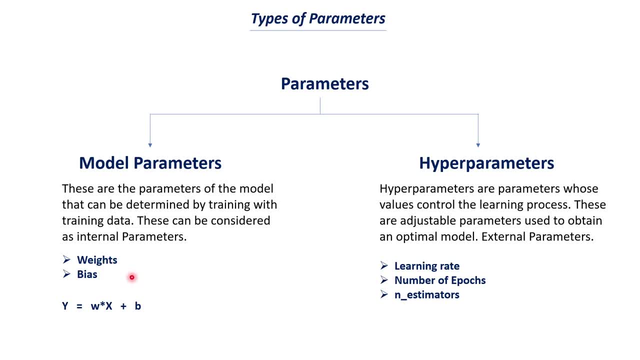 the value of weight and bias and again calculate the loss function and the loss function for that particular weight and bias. so in this case the learning rate determines how much change do you want to give to your weight value and bias value. so this is your learning rate. so if you don't, 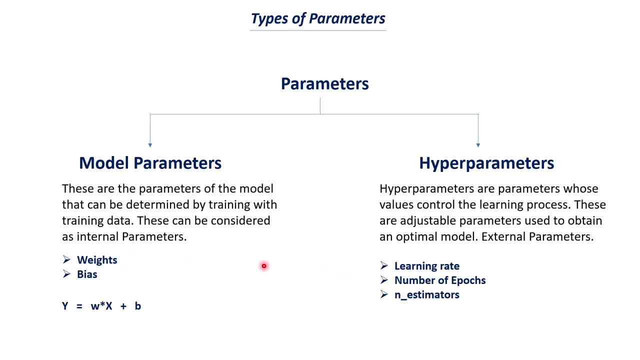 understand this. i'll give the link for my gradient descent video, so please watch that, it will give you a better understanding. okay, so that is an example of learning rate. and then we have number of epochs, so you can also call this as number of iterations. so this determines how many times, uh, you know your. 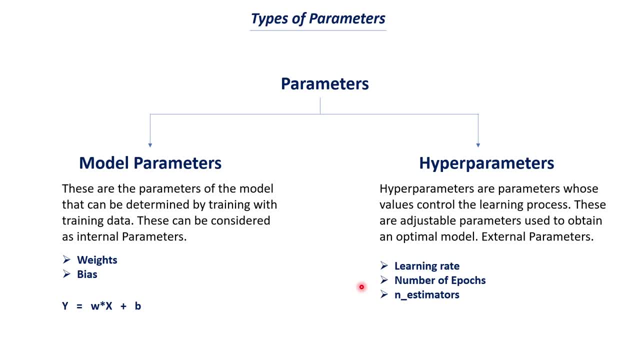 model is going to go through your data. so if you represent this number of iterations as hundred, it means your model will go through the data hundred different times. so you can give it a thousand or whatever you want. so you know, it all depends on how efficient you want your model to be. so if you 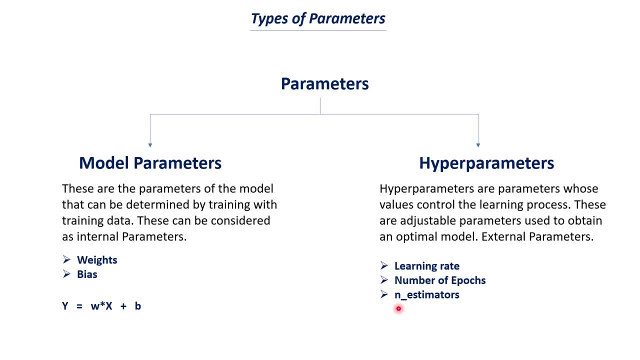 want to use your model to be. and when it comes to a random forest model, there is an hyper parameter called as n estimator. so n estimator is nothing but the number of decision trees that you want in your random forest. so i hope you know that random for is nothing, but it is an ensemble models where 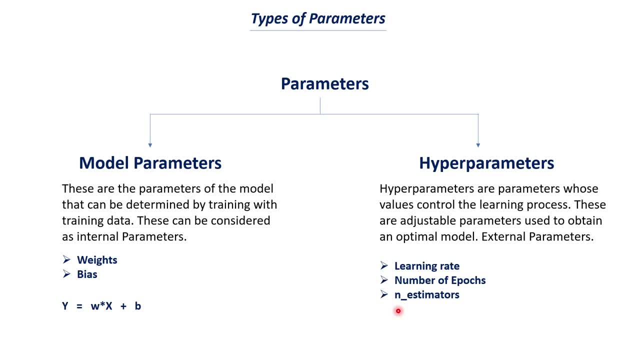 we have several number of decision trees. okay, so it is a group of decision trees and this n estimator is nothing but the number of decision trees we want in our, in our random forest uh model. okay, so these are the two set of parameters. one is the model parameters and the other set of 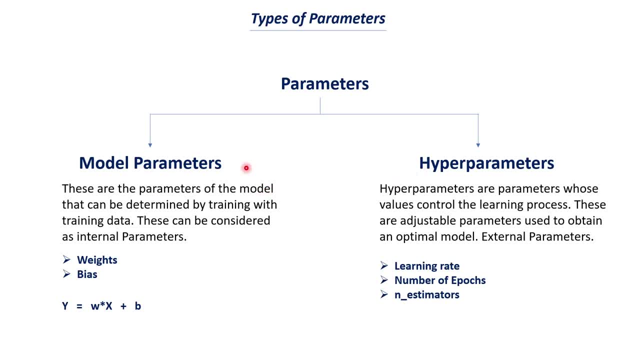 your hyper parameters and the most important thing that you need to remember is that model parameters are derived by the machine learning model by going through the data, by understanding the data, whereas this hyper parameter, uh, hyper parameters- is going to determine how your model is going to train. okay, so these set of parameters, we can change, uh, depending on our requirement. okay. 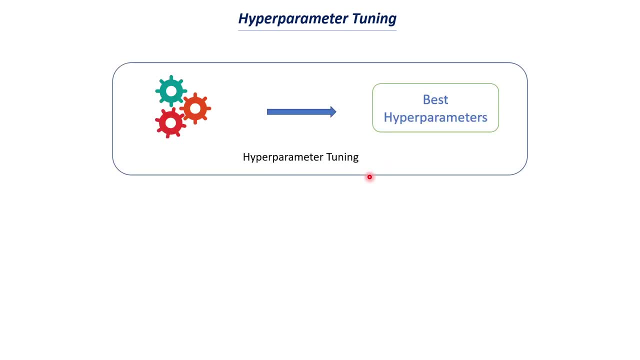 so when we talk about machine learning, these are the two main step. one is the hyper parameter tuning and uh, the next one is the model training. so when we talk about hyper parameter tuning, we try to find or we try to set the optimum value for the hyper parameters, as a you know, as we have. 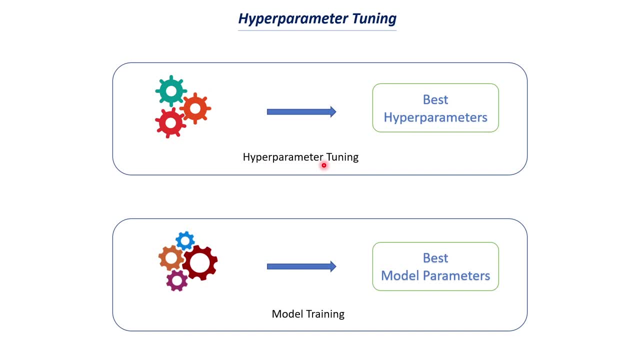 discussed before, the hyper parameters such as number of iterations and, uh, you know, we have the number of epochs and estimators, etc. right, so we will try to uh set, uh you know, optimum values. optimum values is nothing, but for that particular set of hyper parameters you will get the highest. 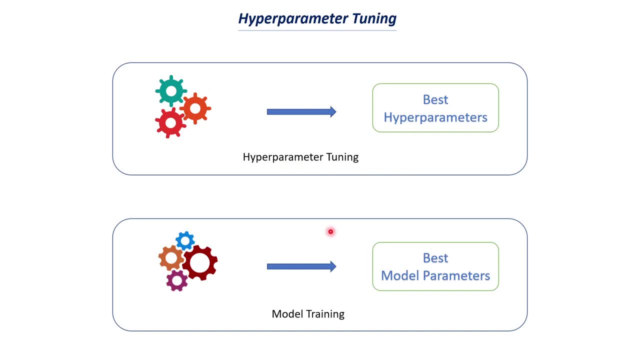 accuracy or is you know, efficiency for that particular machine learning model and model training. so model training is, in this case, you know we uh may implement a lot of the algorithms, like uh gradient descent, which is an optimization algorithm that will try to give you the optimum weight value, bias value and other model parameters value. so the main important, 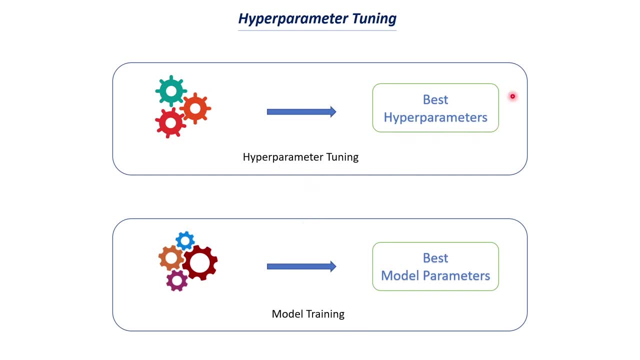 task in machine learning is to carry out these two steps so that we can get the best hyper parameters and the best model parameters, and the reason for doing both these things is to get the highest accuracy or to get the highest efficiency when we work on machine learning. okay, 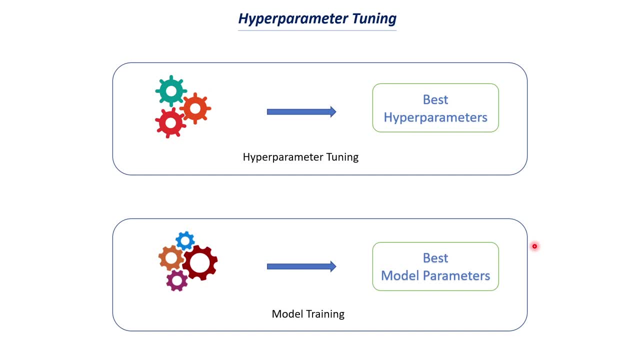 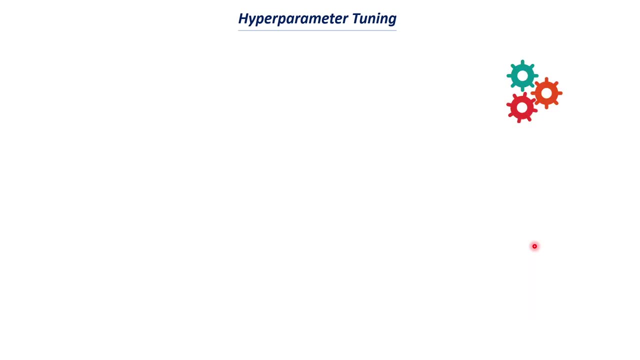 so, as i have told before uh, in hyper parameter tuning we have two main important techniques. so we will try to understand about these two main important techniques, which are cv and randomized search cv. okay, so before uh moving on to that part, i'll just give you a. 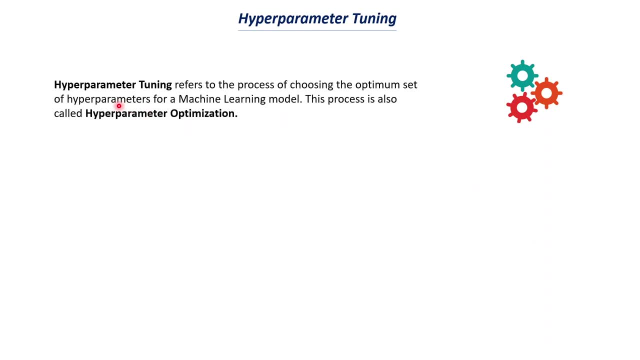 quick definition on what is meant by this hyper parameter tuning. so hyper parameter tuning refers to the process of choosing the optimum set of hyper parameters for a machine learning model. this process is also called as hyper parameter optimization. i hope now you understand the definition of this hyper parameter tuning, as we have discussed this before or in the previous. 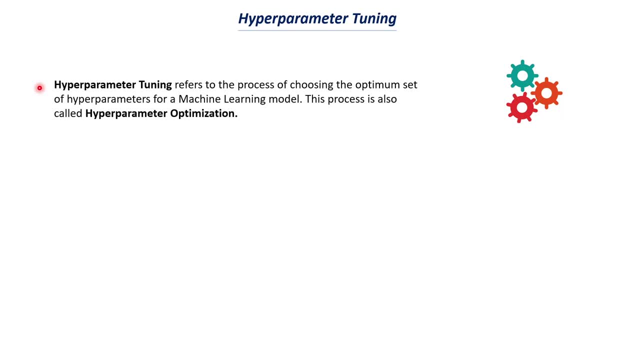 slides. okay, so what we are doing is we are just tuning the hyper parameter values so that we can use optimum set. in the sense we are going to get is accuracy for our machine learning model. so it's not like we are going to do this for only specific model. so it's not like that we will do. 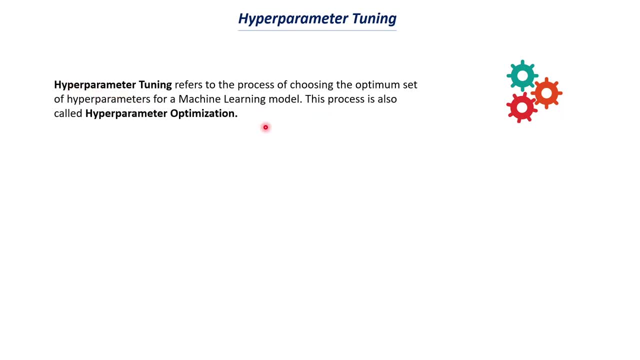 this for all the machine learning models that we will work on. okay, and this, you can also call this as hyper parameter optimization, because we are just optimizing the process of, uh, you know, training the machine learning model by these set of parameters. and again, there are two types of. 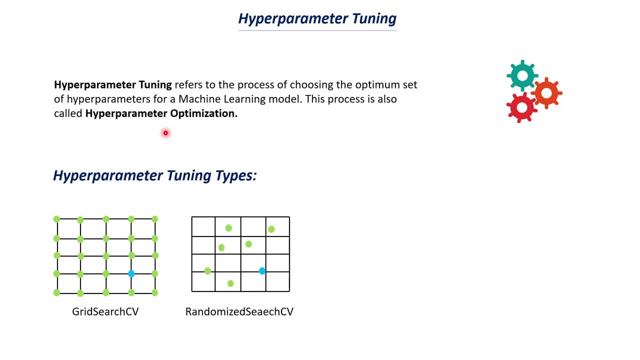 hyper parameter tuning. one is grid search- cv, and the another one is randomized research- cv. okay, so what we will do is so, uh, when we have a machine learning model, when we take a machine learning model, there are different and hyper parameters that we need to work on. okay, and there can be. 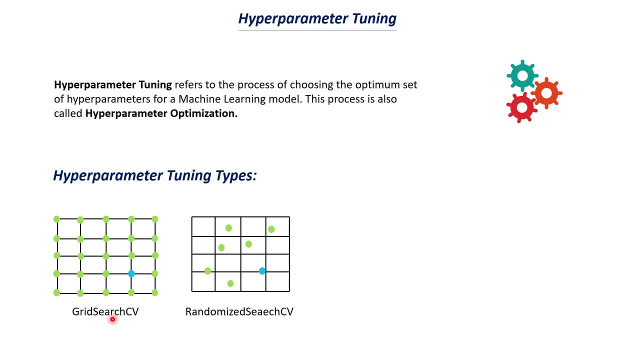 different possibilities, different values that hyper parameter can take. so when we uh use a grid search- you know, use a grid search, cv technique- we will try to uh, you know, use all those values. so we will, in each time we will try to uh check that particular hyper parameter value and see. 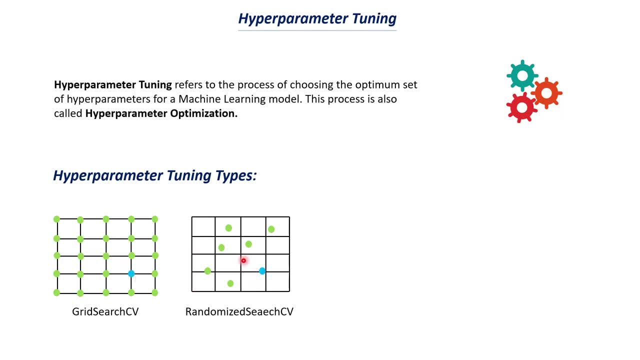 which value is giving us the highest accuracy. and in the randomized search, we, instead of uh calculating uh the performance of the model for different combinations of hyper parameters, we will randomly select only few parameters and then we will try to find which is the best value. okay, so here, blue color dots represents the best value and the green color uh. 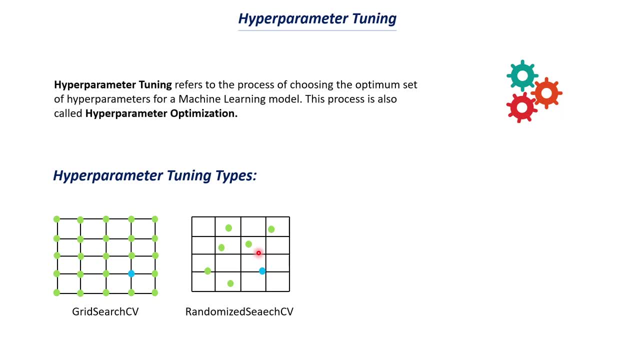 you know, dots represents the different uh hyper parameters values which you know we can choose from. so if you don't understand this, it's completely fine. i'll just give you an example now you will be able to understand this clearly. let's take an example of a support vector machine. 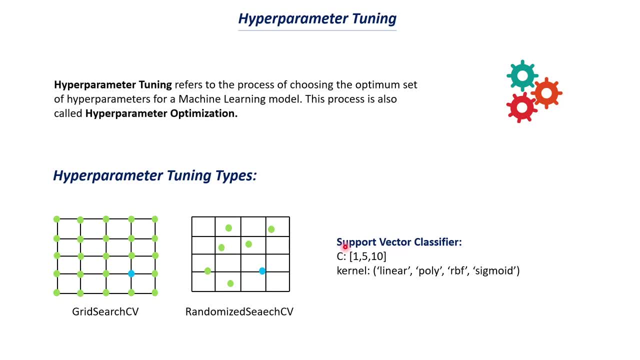 classifier. okay, so we know that this is a very important classification model that we will work on in machine learning. so examples of uh hyper parameters for support vector: uh machine classifier includes c value and kernels. okay, so c is nothing but uh, you know what is the penalty that you are setting for your model. so if your 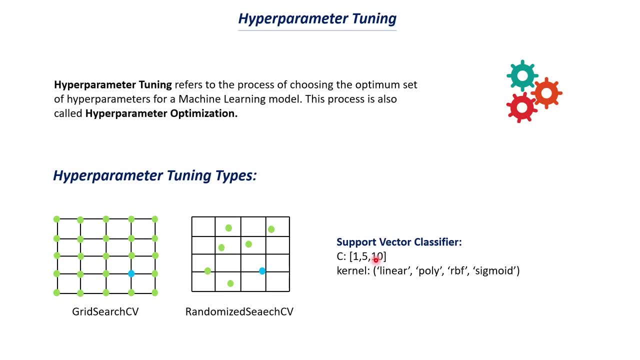 c value is very high, that means your model doesn't allow any misclassifications, okay, whereas if your c value is, uh, very low, that means, like, your model allows some misclassification to occur. so this is the importance of c value. so i value of c means no misclassifications are allowed for the two classes, or three classes, that you are. 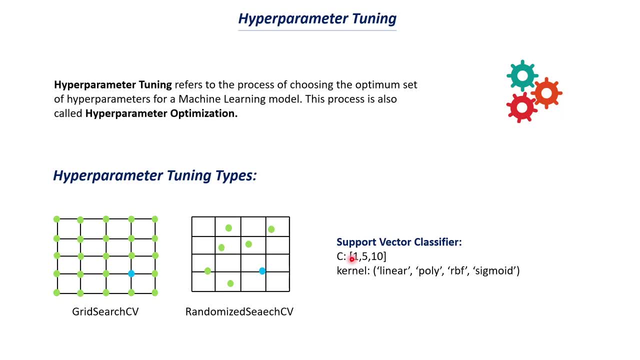 working on, whereas low value means you can have misclassifications. okay, and kernel is. you know, we have discussed about this in our support vector machine classifier, so we have built the support vector machine classifier from scratch. so in that thing i have explained you how this linear. 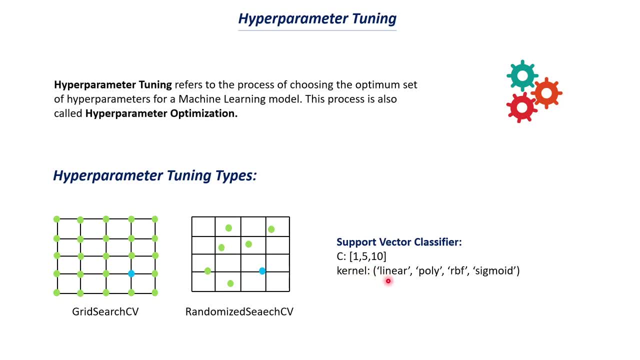 polynomial kernels. everything works, so i'll also link that video as well. in this video description you can check that out. okay, so these are all different possible values that you can have for your c and kernel. okay, so now let's try to understand this grid search, cv and randomized. 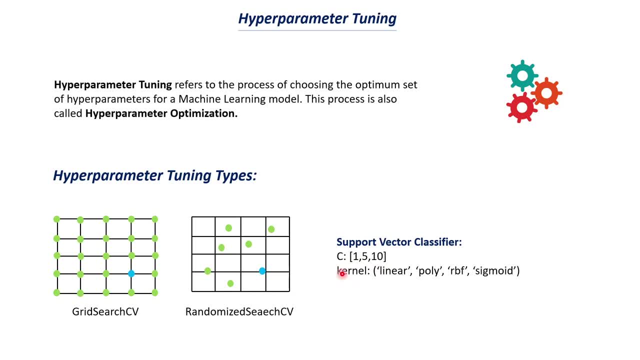 search cv based on the support vector machine classifier. okay, so in this case, we have three set of values, right? so what we will do is we will, uh, create a list or we will, you know, mention. so these are all the possible values that i want to check, and we just want to check for which values. 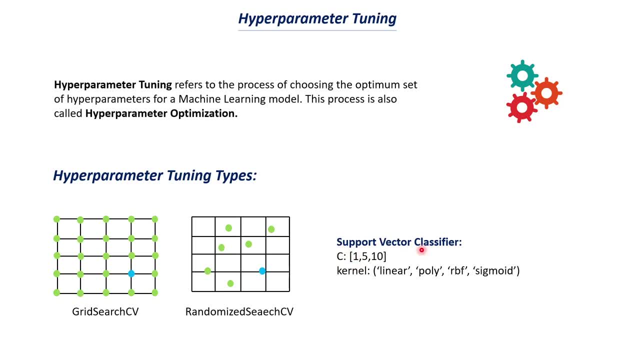 of c we are getting i accuracy when we are using a support vector machine classifier. similarly, we have different kernel values, so we have linear kernels, polynomial kernels- rbf basically means radial basis function kernels- and sigmoid kernels. so these are all the different set of kernels we have. so we need to check for which combination of c and kernel values we are. 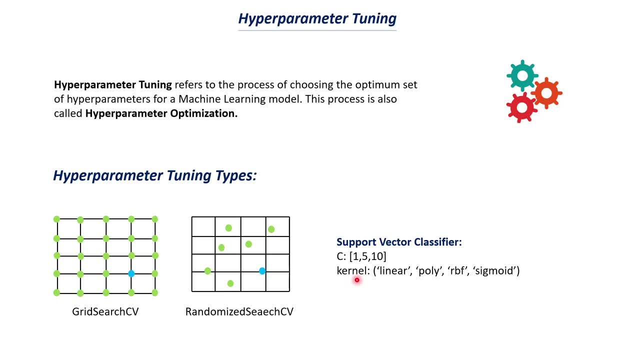 getting the highest accuracy for that particular data set. okay, so here, green color dots represents the different possible values that we are going to take and blue is the value with, you know, highest accuracy. let's say that for c value of 10 and the kernel value of polynomial, let's say that we are. 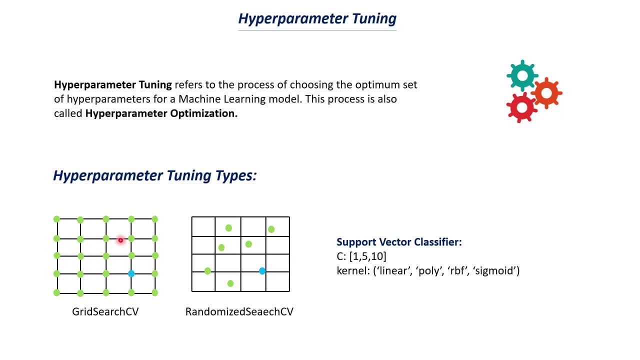 getting highest accuracy. so that is represented in this blue color dot. okay, so this is just a graphical representation of understanding grid search cv and randomized search cv. okay, so in this case. so green colors, you know, dots represent all the values that we are going to test and 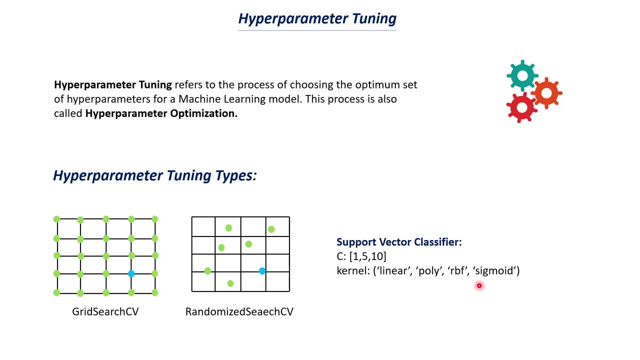 in this case we are just taking three values. okay, and for kernel we are taking four values. so out of all these values, which is your best value? so we will consider each value for the c and kernel and then we will try to find this accuracy and finally we will choose the hyper parameter value. 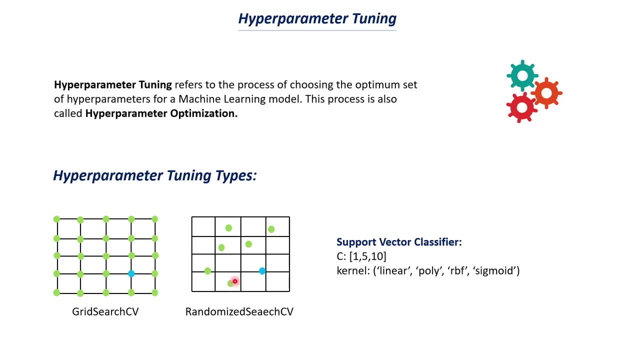 for which we are getting highest accuracy, which is represented in this green color, and uh, so this is not doable and this is not. you know, we can't, you know, do it every time we are working on a machine learning project. the reason is that you can have a several number of possibilities. you can have several combinations of the c.